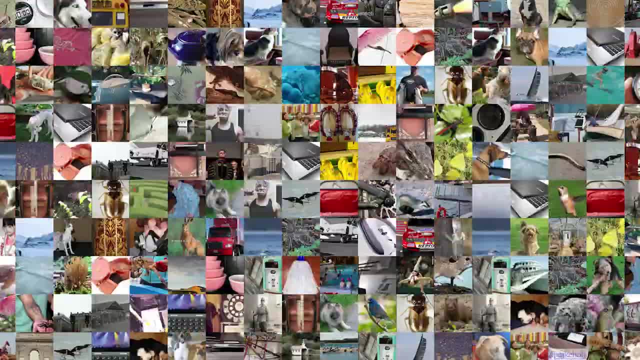 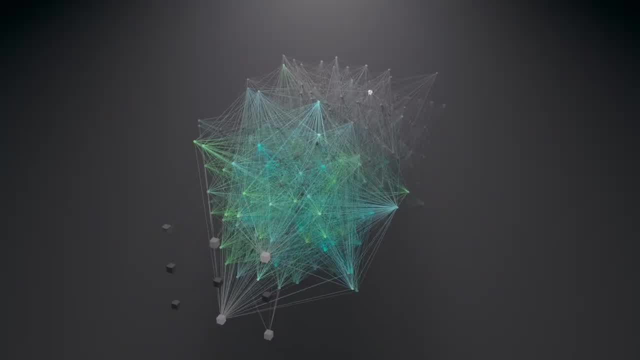 There's a whole other traditional model on this large database called ImageNet, So there's really no better tool to use. Neural networks are computing systems that process data in ways that mimic the human brain, And when using machine learning and neural networks, there is one resource valued: 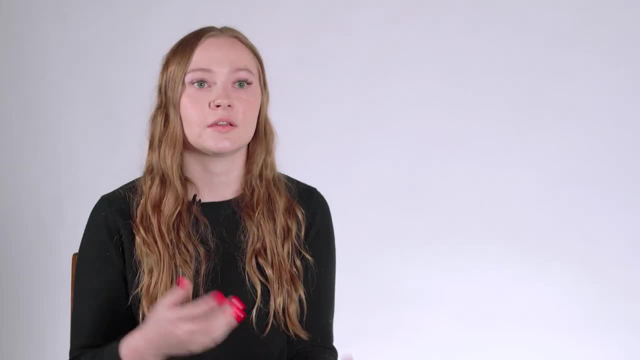 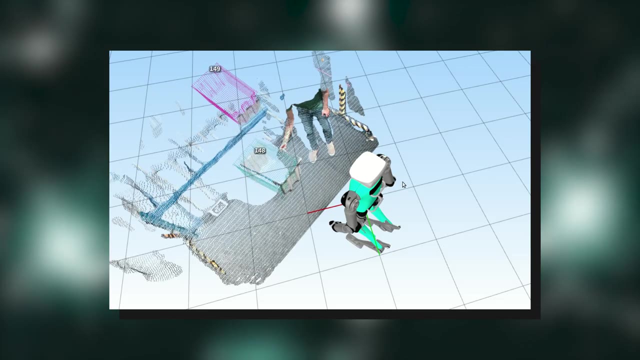 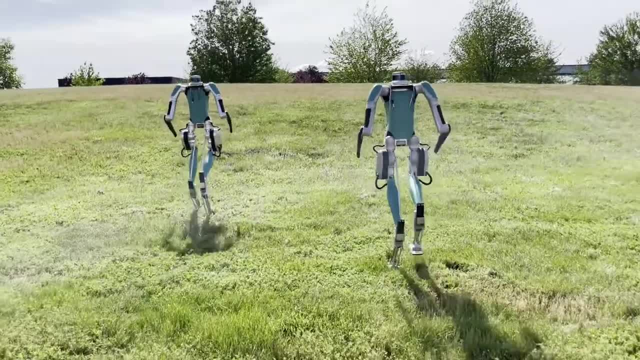 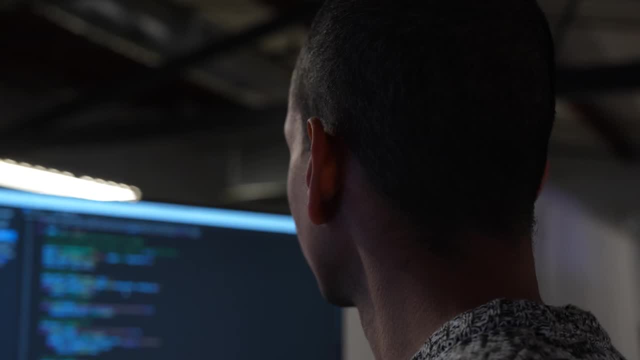 model in a certain environment And we deploy in a different environment. that's going to really start to challenge our perception algorithms. Currently, perception algorithms require lots of human intervention and maintenance and they are mostly tailored to specific tasks. Engineers have to manually filter through. 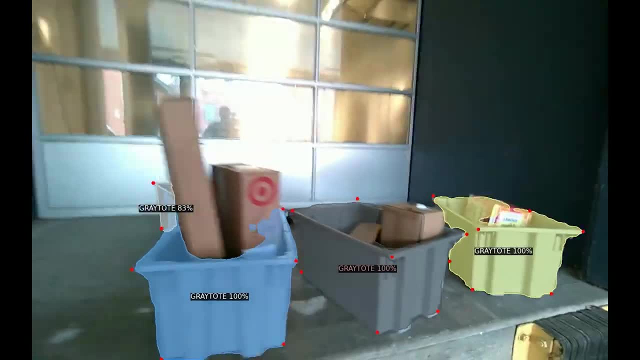 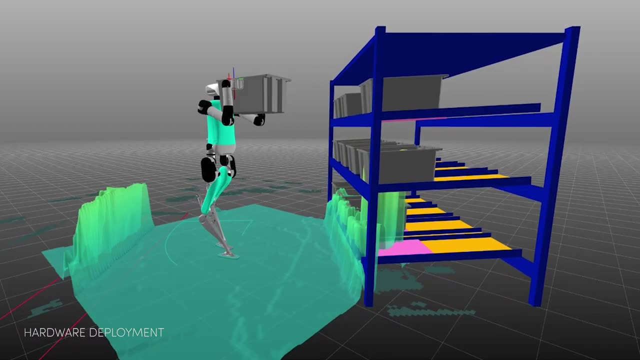 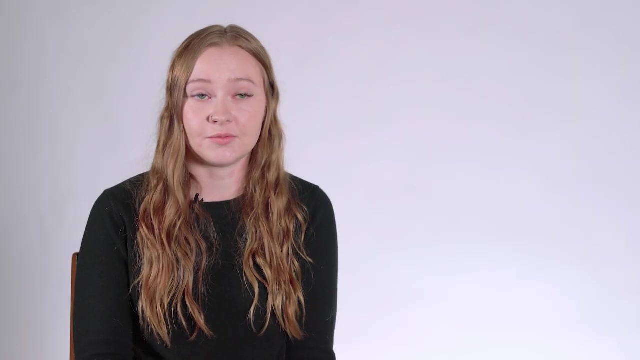 training data to help teach the model what's what. But the world isn't predictable and it isn't easily modeled. It's full of randomness and uncertainties. So general purpose robots will need to be able to adapt on the fly. We try to show the models as much as we can of variation. that's even unrealistic, so that 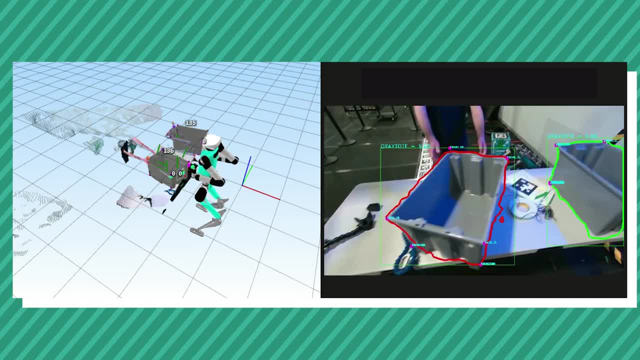 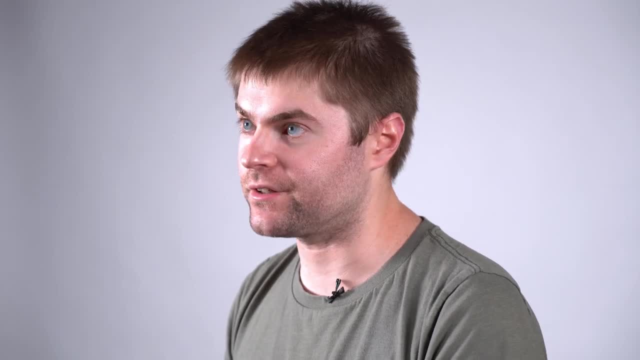 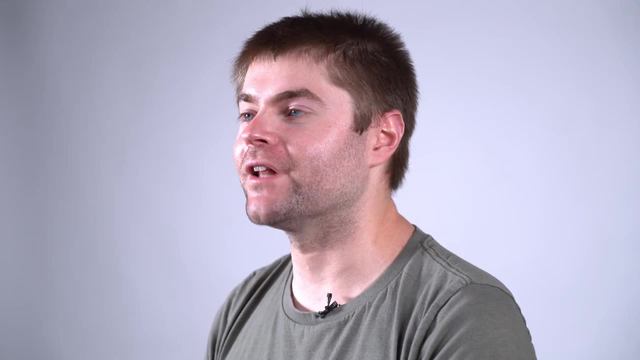 it can generalize to a good point. Instead of developing a perception algorithm to run once on one set of data, you want to be developing an algorithm that's robust to unseen scenarios. One thing that we're constantly thinking about is identifying those cases where the perception algorithm fails: filter. 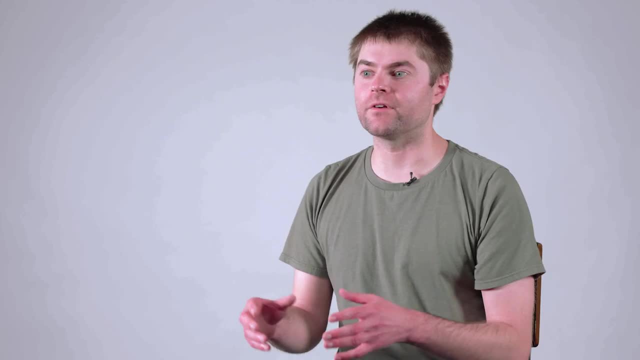 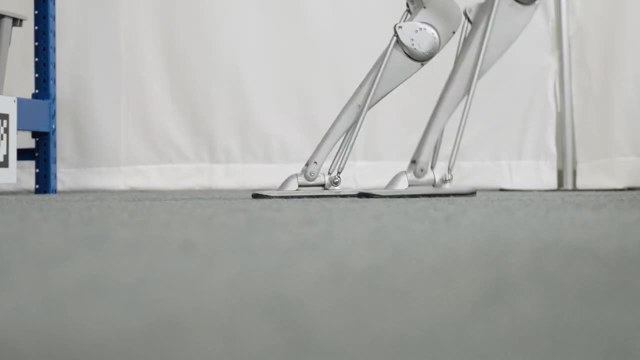 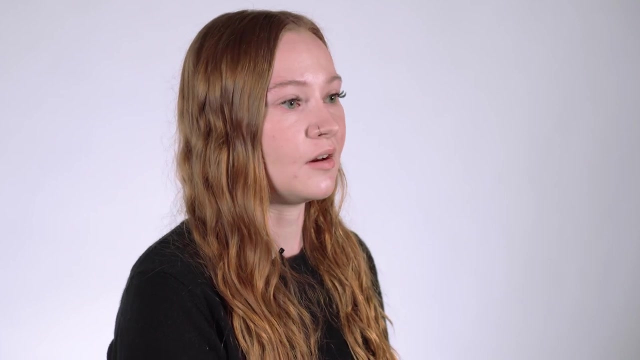 that information back to the engineers And then we can design different algorithmic solutions for that. The goal is that someday robots will be able to do this themselves, using their onboard systems to detect failures and make corrections. We have so much complexity, so many things that come into play and we want Digit to 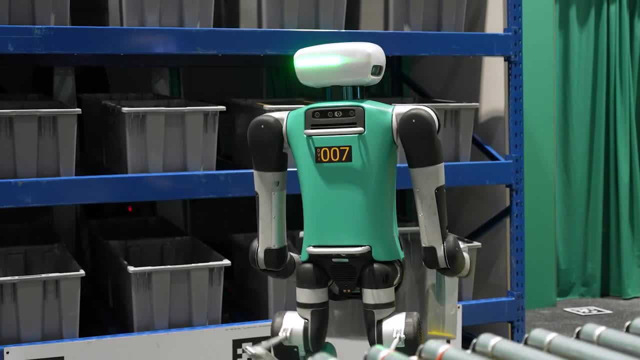 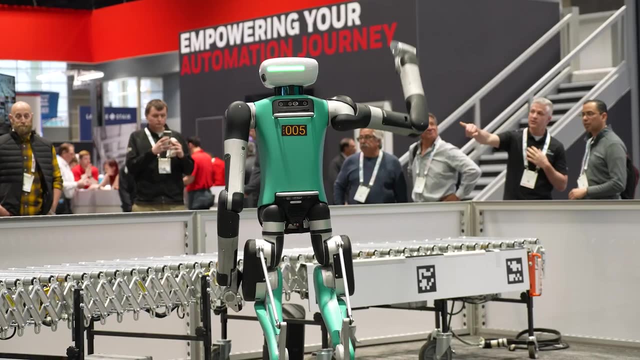 be able to interact with all of those things and handle them dynamically, handle people in situations and totes in unknown locations, things like that- and be able to still do its job safely. Subtitles by the Amaraorg community.